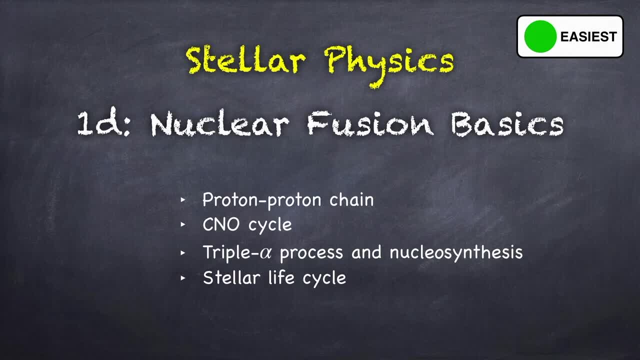 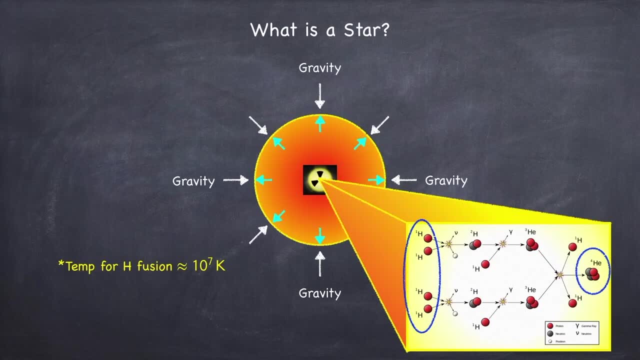 so that when we get into the detailed physics inside of stars, we'll be able to place it inside a greater framework of the stellar life cycle. Recall from previous videos in this series that stars are powered by nuclear fusion in their core that counteracts gravitational collapse. 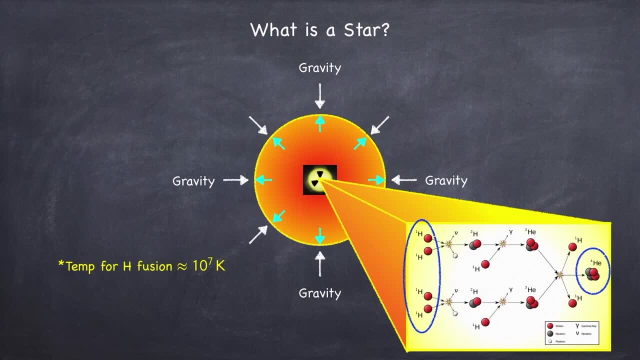 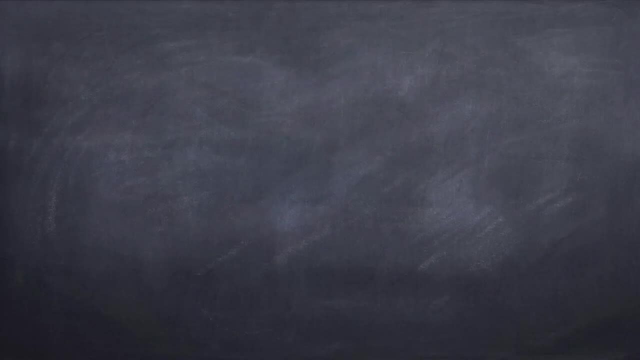 More specifically for what are called main-sequence stars, and we'll see what that is. that fusion is hydrogen fusing into helium. Typically, you need a temperature around 10 to the 7 Kelvin for this to take place. So let's look at the details of hydrogen fusion, starting with the proton-proton chain. 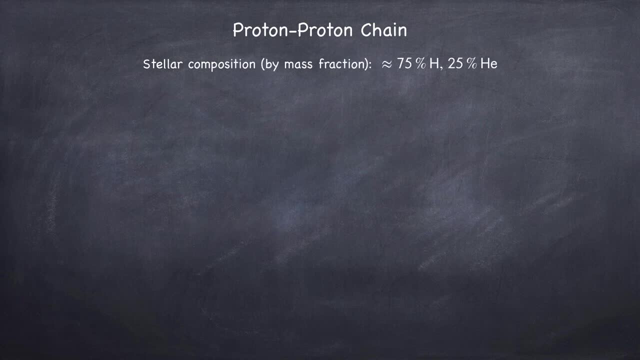 Stars have a stellar composition of about 75% hydrogen and 25% helium. There may be other metals in there, but anything else would be less than 1%. If there are POP3 stars- recall from Physics 1a that would be the first generation of stars- then they have nothing else. 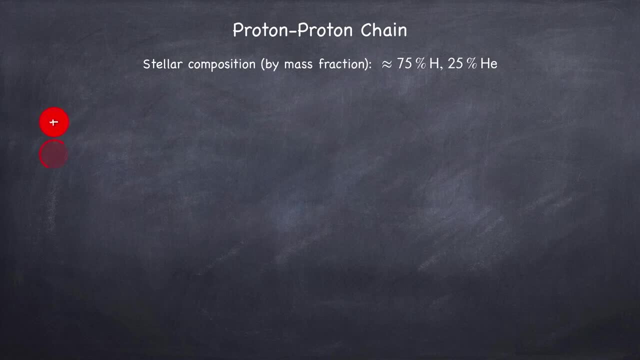 So the way the proton-proton chain works is, if you have two protons or helium nuclei in the star, they will come together and they will fuse into a proton and a neutron. So one of these protons has to convert into a neutron. 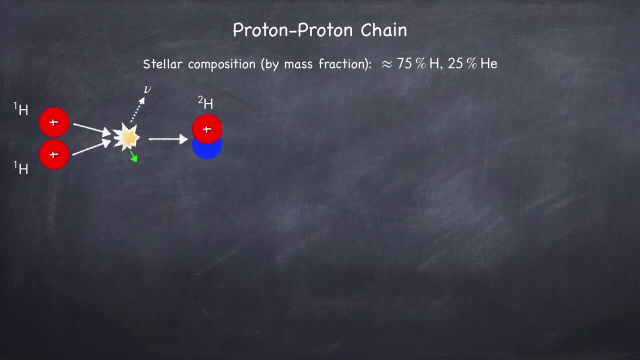 and in the process it will emit a neutrino and a positron. You have to emit a positron because charge has to be conserved And since you've lost charge when you converted one of your protons to a neutron, that's got to go somewhere, so it goes into this positron. 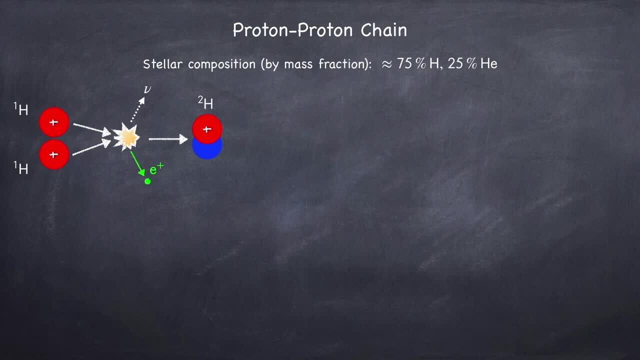 The force that is responsible for this is the weak force, and whenever you have the weak force, you emit neutrinos as well. So when you see a neutrino, you know you're dealing with the weak nucleus, You're dealing with the weak nuclear force. 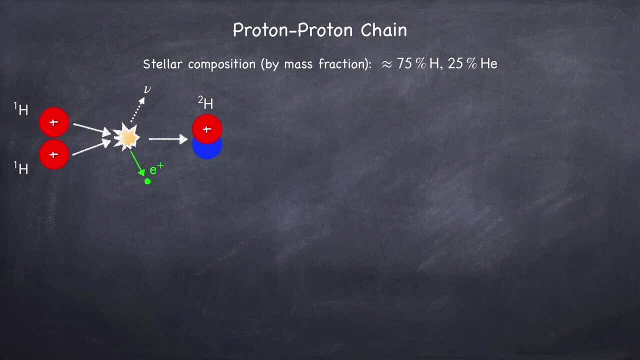 Now, the star is a plasma and it's neutral, so there are as many electrons around as there are protons. so when this positron pops off, it will immediately encounter an electron and those will annihilate into two gamma rays or photons. 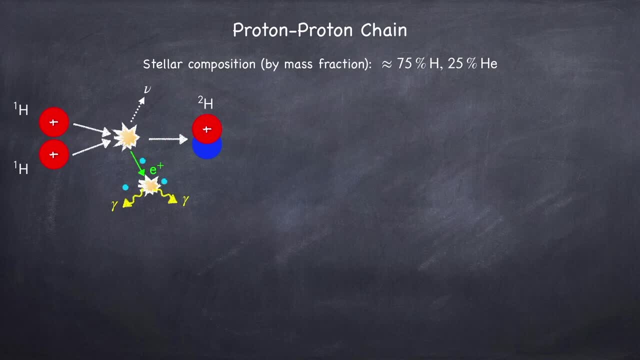 This energy is dumped into the star, whereas the neutrino, as we've mentioned before, just leaves the star, and that's energy lost. Later on we'll see that neutrinos play a larger role, but in this stage they're just lost energy. 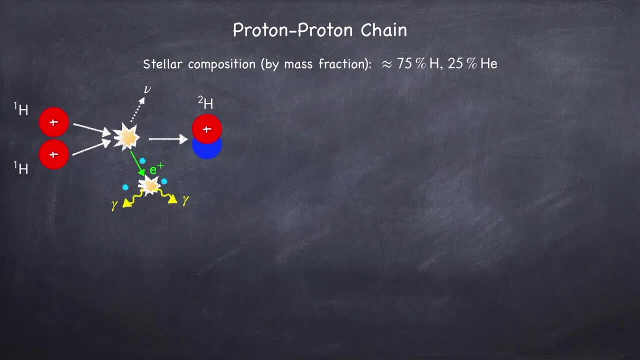 So now we have H2, which is hydrogen with a mass of two, meaning it's got atomic number of two. it's made of two baryons. It's still hydrogen because it still has a charge of one. It will then encounter another proton and those will come together. 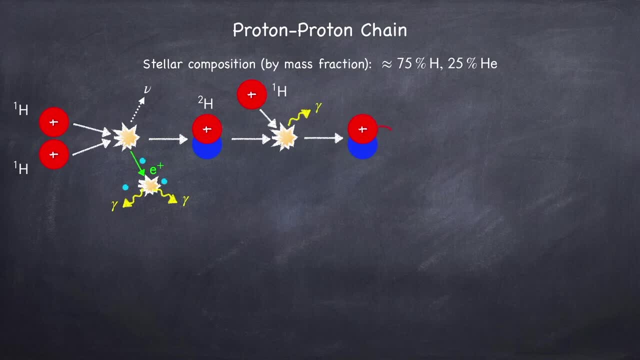 and they'll fuse and emit a photon to make helium-3.. So this is helium because it's got charge two, but it's helium-3, since it's got a mass of three. So here we see, we've already made helium, But helium-3, while it's stable, is not as stable as helium-4.. 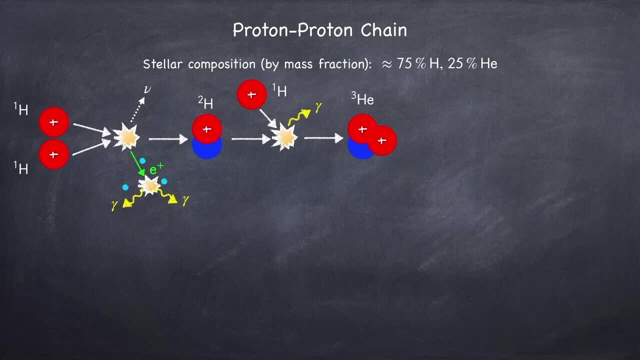 So this would like to be in the form of helium-4.. By the way, the 25% helium that's in the star part of that is already helium-3.. So here we have this branch of the proton-proton chain. 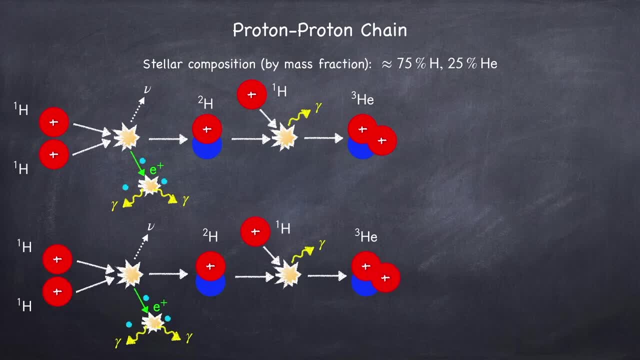 and nearby. the same thing happens with some other protons And now we have two helium-3 atoms or two helium-3 nuclei. So now these two helium-3 nuclei come together and they fuse, They pop off two protons and a helium-4 nucleus or an alpha particle. 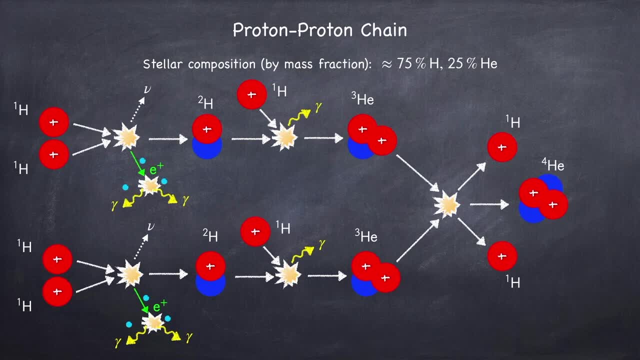 And now we have helium-4. And once you're at helium-4, this will basically stay at helium-4.. Helium-4 is one of the most stable nuclei out there and baryons like to be put into helium-4 nuclei. 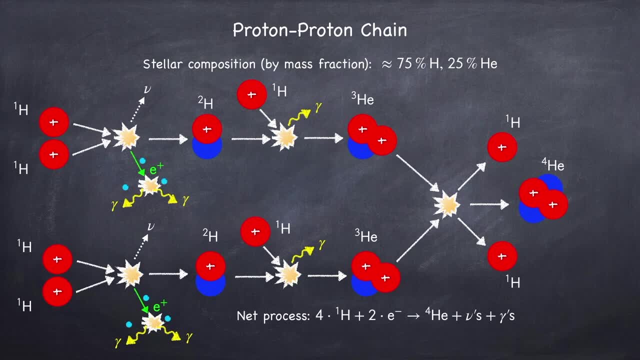 And so the net process is that we have four protons and two electrons come together to make a helium nucleus, an alpha particle, plus neutrinos and photons. The total energy released is simply the energy corresponding to the mass difference between the initial particles and the final particles. 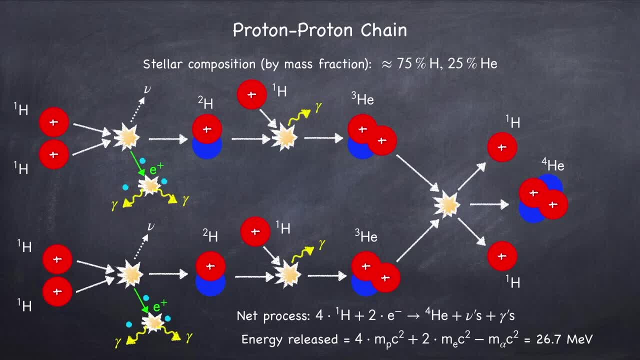 And that comes out to 26.7 mega-electron volts. Now notice here I didn't show any photons or any other particles being emitted in this process. That's because there need not be one In this case. all of the binding energy between the helium-3 nuclei and the helium-4. 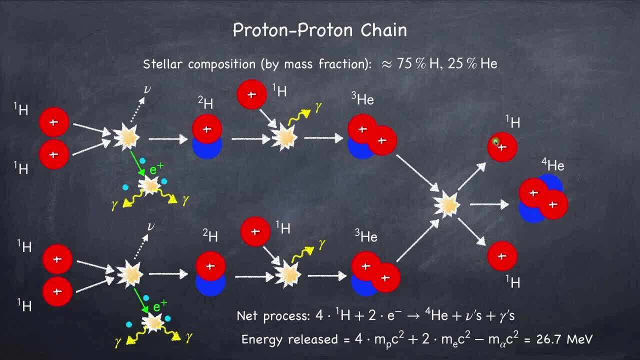 could go entirely into kinetic energy, Or it could go into a photon. They're completely interchangeable, as photon number is not a conserved quantity. In this case, however, when you take the deuteron and the proton, here you have two nuclei coming together and sticking together and making one nucleus. 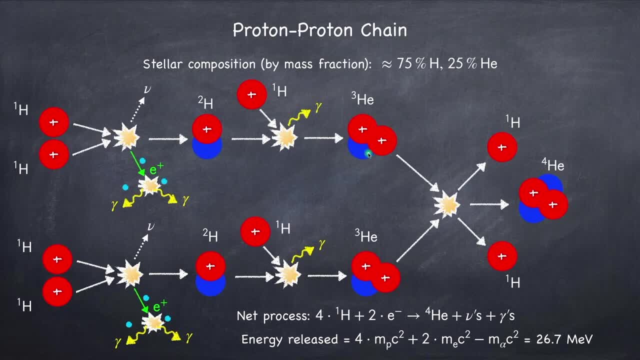 So this is a completely or a perfectly inelastic collision, and so energy is not conserved. It's impossible for energy to be conserved, So that energy has to go somewhere else. so you have to emit a photon to account for that missing energy. 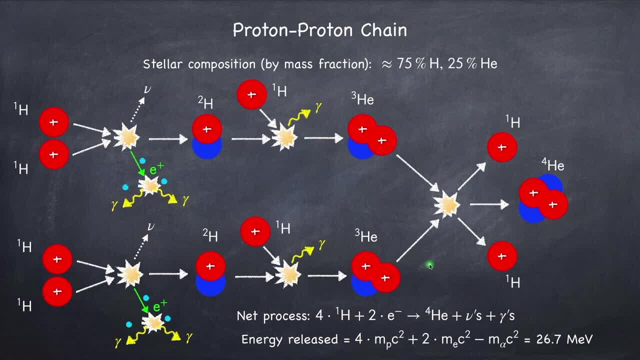 So this branch here, this is sort of the main branch of the proton-proton chain. there's all sorts of other branches and combinations that can take place, but you get the basic idea. They all result in four protons being converted into a helium nucleus. 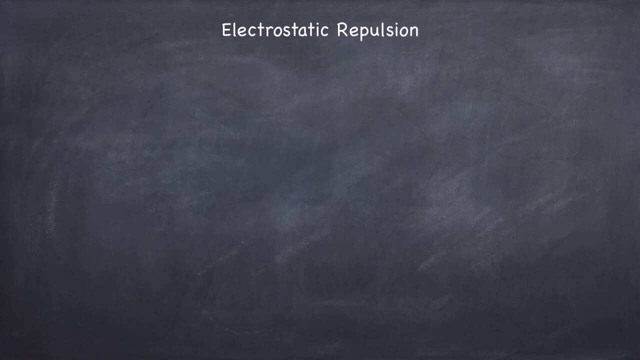 Now there's a problem here. Protons are positively charged, so they want to repel each other due to the electrostatic force or the Coulomb force. So how do they come together in the first place? Why do they stick together? 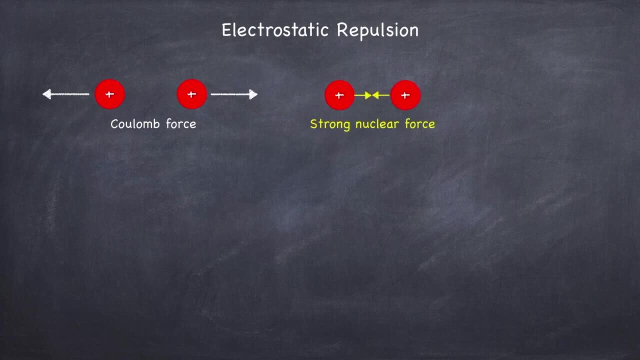 Well, they stick together due to the nuclear force- the strong nuclear force in this case, that is stronger than the electric force at close range. When they're far apart, the Coulomb force wins, but if they're close enough, then the nuclear force wins. 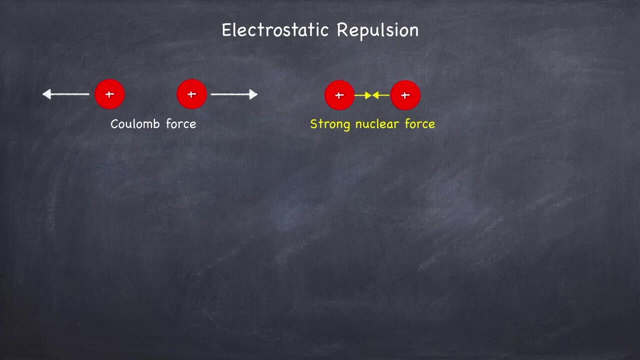 The nuclear force is much stronger at short range, but is weaker at long range, Or the strong nuclear force, I should say. So how close do these have to be before they stick together? Well, they have to be. at about a nuclear radius. 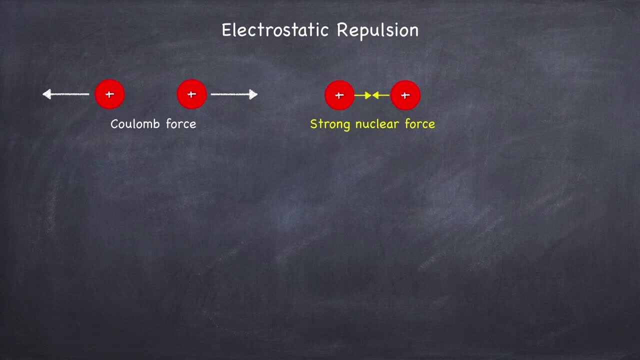 Which is about 10 to the minus 15 meters. So how do these protons get close enough in the first place? Well, they have to be moving very fast. Just how fast they have to move? Well, when they get to the closest point. 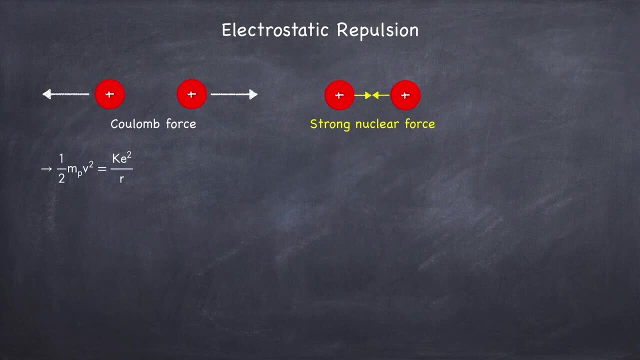 all of the kinetic energy will have been converted into potential energy. So if we take a frame in which one proton is at rest, the kinetic energy of the other proton will have to equal the potential energy at the closest point. So Ke squared over R is the 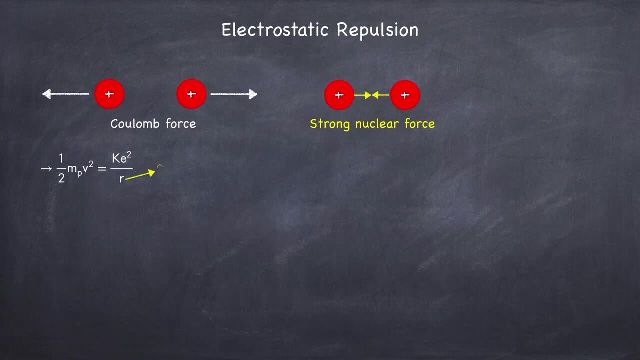 electric potential energy at a distance R which we are going to set to a nuclear radius K. here is Coulomb's constant. We can now solve for the minimum velocity and find that it's about 10 to the 7 meters per second. 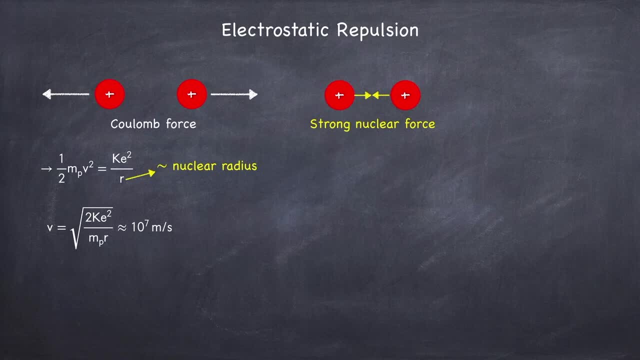 or 10,000 kilometers per second. Naively, we might just try setting this to the average velocity, and since we know that the average squared velocity is related to the temperature, if we square 10 to the 7 meters per second, 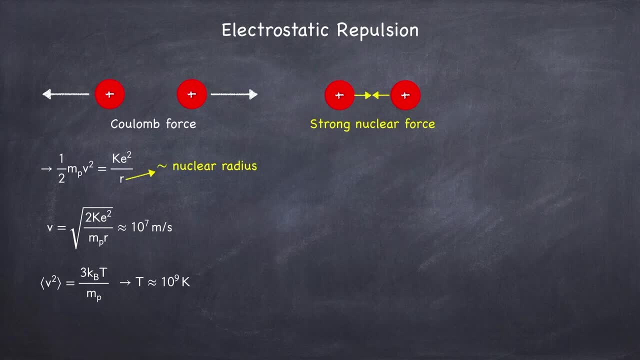 this gives us a temperature of about a billion Kelvin, But you may recall that I said you only need a temperature of about 10 to the 7 Kelvin. So why is that? Let's take a look at a Maxwell-Boltzmann velocity distribution. 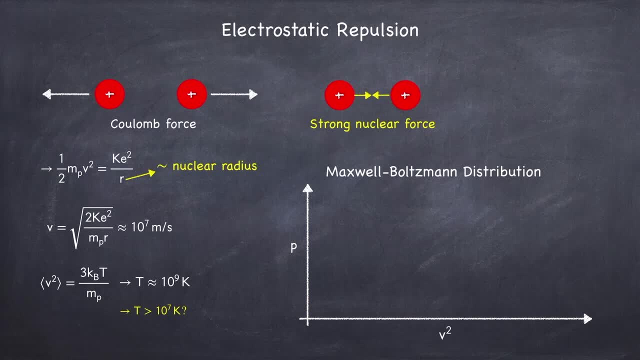 On the x-axis I have the velocity squared and on the y-axis I have the probability of having that velocity, And the graph will look something like this, where the average squared velocity will be around here somewhere, And that's what's related to temperature. 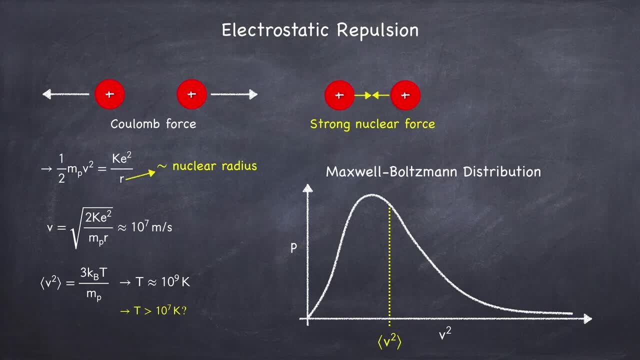 But not all protons will have that velocity. Even if the average squared velocity is about 10 to the 7 meters per second, out here in the tail you'll have much higher velocities, So you don't need the average proton to have a high enough velocity. 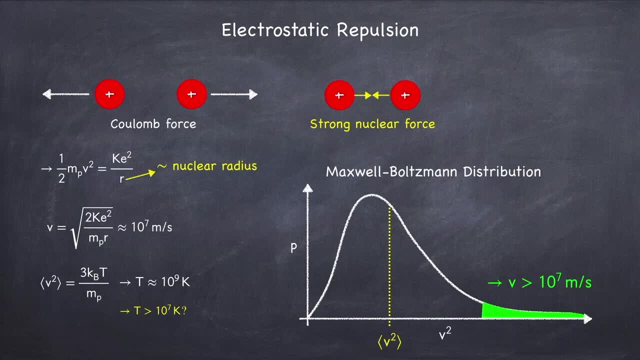 to overcome the Coulomb force as long as you have enough high-speed protons in this tail to produce enough energy to overcome gravitational collapse. And it works out that at about 10 to the 7 Kelvin you'll have enough. This depends somewhat on the mass of the star. If the mass is larger, gravity is stronger, so you need a higher temperature, So small stars are colder than large stars in general. Now let's take a look at the CNO cycle. This is another way in which hydrogen can fuse into helium. 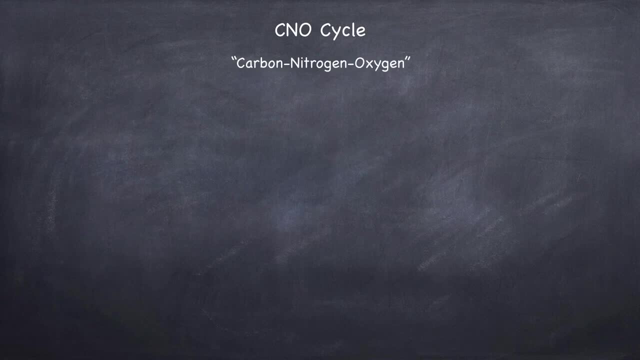 And CNO stands for carbon-nitrogen-oxygen. So for this to take place, you need to have some carbon-oxygen-nitrogen-oxygen And you don't need a lot Recall. I said: everything other than hydrogen and helium is less than 1% of the star. 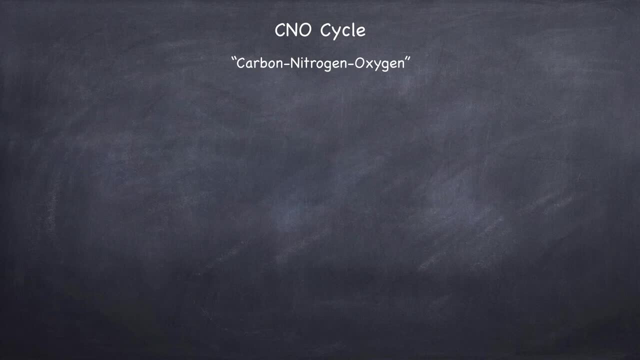 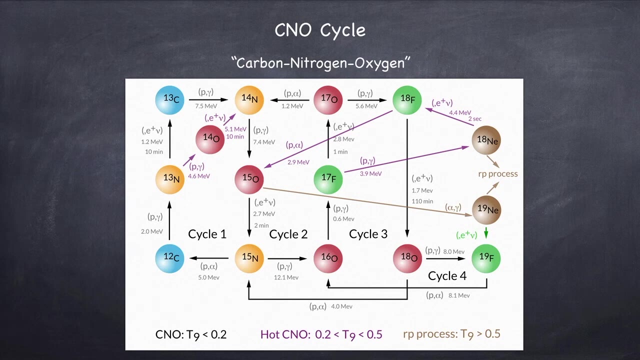 Also, you need slightly higher temperatures. So here's a schematic of the CNO cycle. It looks pretty complicated and there's numerous branches. I'm just going to go over cycle 1 here. The other cycles are the same idea. You can pause the video and take a look at them. 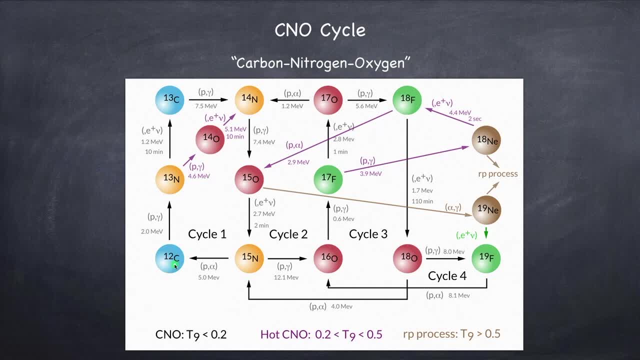 if you want to see in more detail, Recall: all these nuclei make up less than 1% of the star and they're surrounded by a sea of hydrogen and helium. So we start off with carbon-12, and we capture a proton to make nitrogen-13. 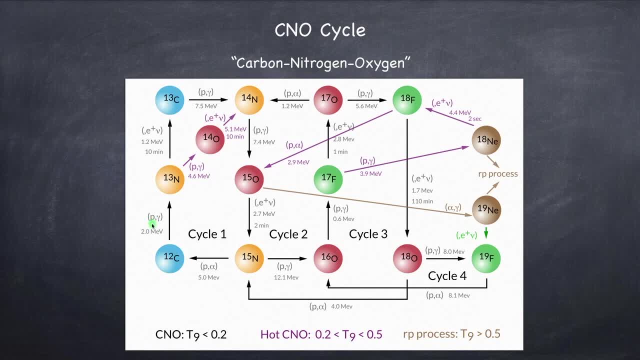 The way to read- this is the first entry here in the parentheses- is what's being captured. So we have a P for proton and in the process we emit a photon, and here it tells us how much energy is released. So here we've captured a proton. 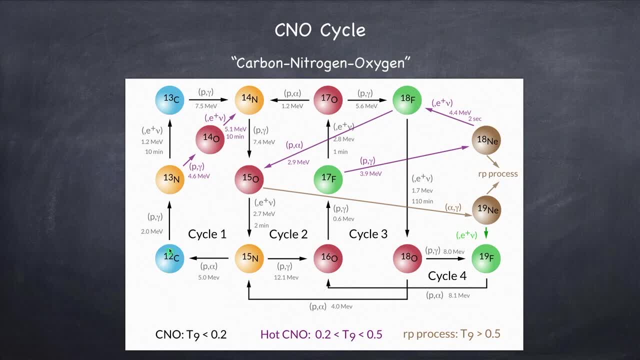 which increases the charge and the mass by 1. So by increasing the charge we go from carbon to nitrogen. It's a new element And we've increased the mass by 1, so we go 12 to 13. So this is nitrogen-13. 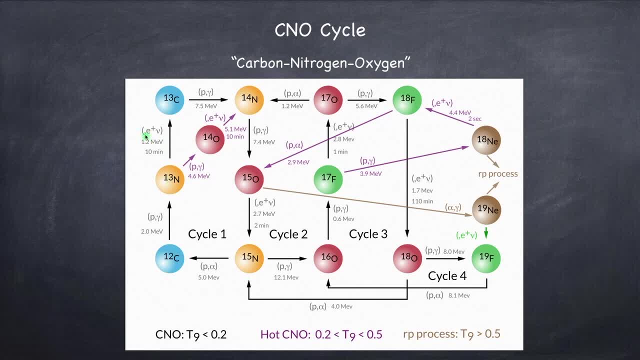 Then we have a beta decay. So that's what's going on here. You see, nothing's being captured. We just emit a positron and a neutrino Electrons and positrons are also called beta particles, So this is called beta decay. 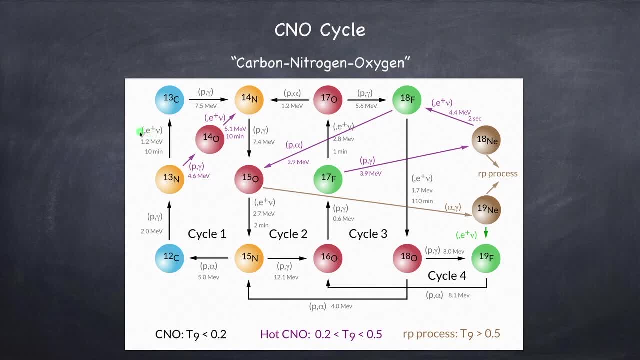 So since we've lost a charge but we haven't emitted any baryons or captured any, we're still at 13,. but we're back down to carbon, So we have carbon-13.. Then that captures another proton and emits another photon. 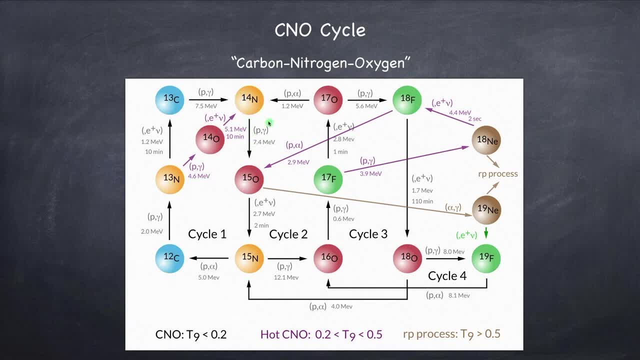 to make nitrogen-14.. We again capture another proton and emit a photon and we make oxygen-15.. Then there's another beta decay, so we're going to lose another charge, So we have nitrogen-15. And then finally, we capture a proton. 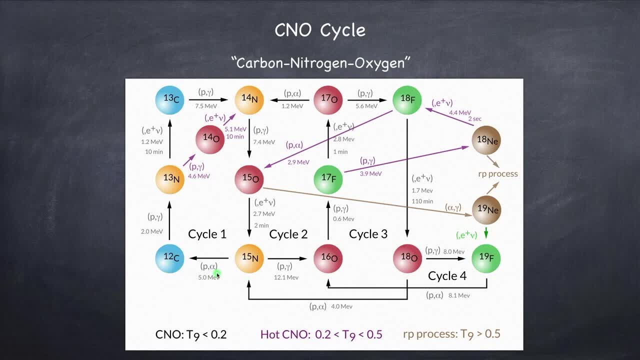 and emit an alpha particle, And so we've made helium, And then you repeat the cycle again. Now here. you could have gone a different way. You could go into cycle 2 by capturing a proton and emitting a gamma or a photon. 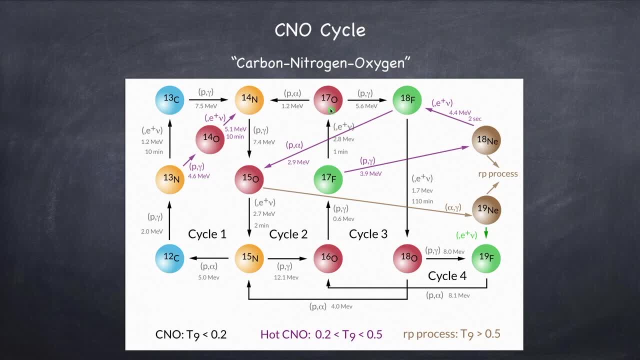 instead of emitting an alpha particle, And then you're in cycle 2, which up here will branch either back into this branch here- Notice, here we've captured a proton and emitted an alpha particle, so we've made helium again- Or you can go this way into cycle 3,. 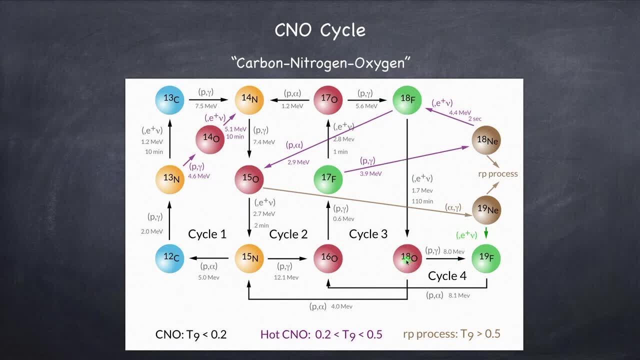 which then branches to cycle 4. this way, And in cycle 3, you make an alpha particle here, Whereas cycle 4 makes your alpha particle there. And which way you branch, both will happen at the same time, Just with different probabilities. 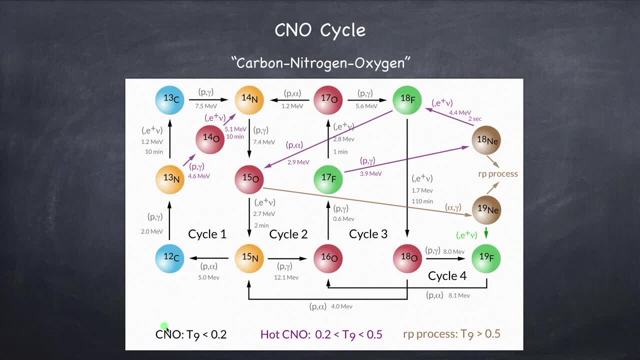 So what's the difference between these black cycles and these purple and this brown one here? So the first one is called the cold CNO cycle or the regular CNO cycle, And this T9 here means a temperature in units of 10 to the 9 Kelvin. If the temperature is less than 0.2 times 10 to the 9 Kelvin, the cold CNO cycle will dominate. It doesn't mean you don't have the hot CNO cycle happening as well, It's just the dominant one is the cold CNO cycle. 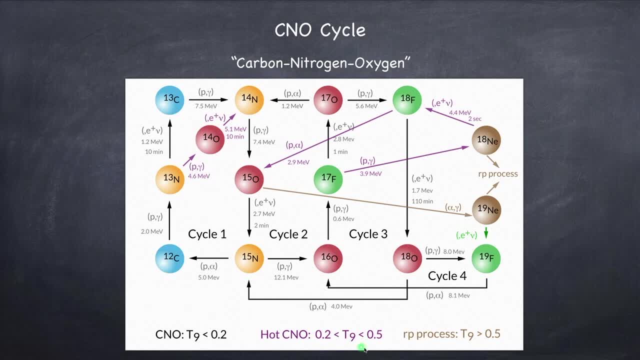 Above T9 of 0.2 and below 0.5, the hot CNO cycle will dominate And if it's really hot, higher than T9 of 0.5, what dominates is called the RP process, which stands for rapid proton process. 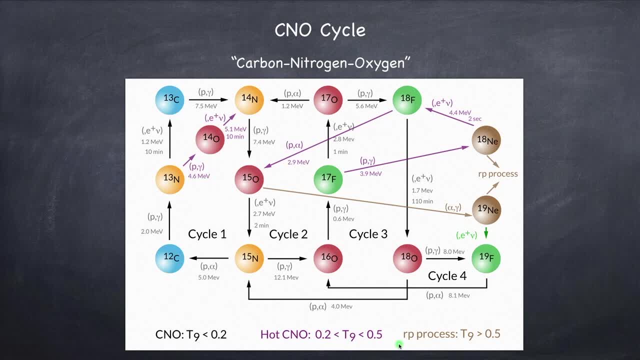 And this is when the material is so hot and the protons are moving so fast that they just capture on any nuclei that's around and make heavier elements. If you're finding this video useful, please be sure to like and subscribe and maybe share it with a couple friends. 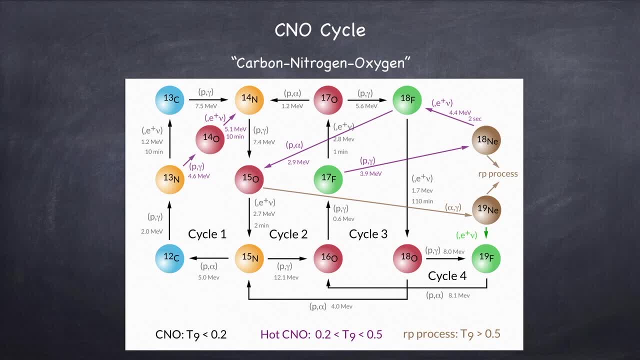 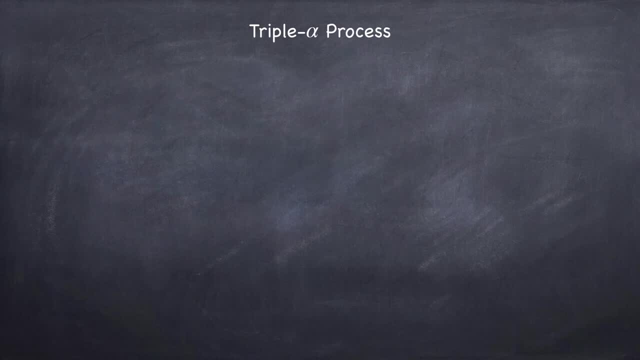 So that basically covers everything for hydrogen fusion. The next stage in nuclear burning is called the triple alpha process, and this is helium fusion. Eventually all of the hydrogen in the star's core will have fused to helium. At this point the star will have a helium core. 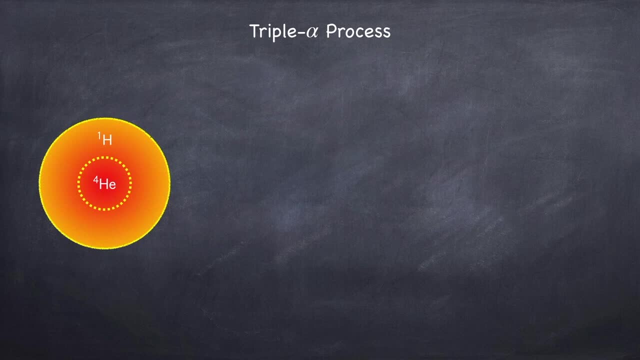 and the outer layers will still be made of hydrogen because they weren't hot enough for fusion. Since there's no more hydrogen to fuse in the core, there's no more energy to support it against gravitational collapse, and the star will start to contract. As it contracts, it will get hotter. until it's hot enough to fuse helium. Once helium fusion kicks in in the core, the outer layers of the star will get pushed out, they will expand and they will cool off and they will get redder in color, And so this stage is called a red giant. 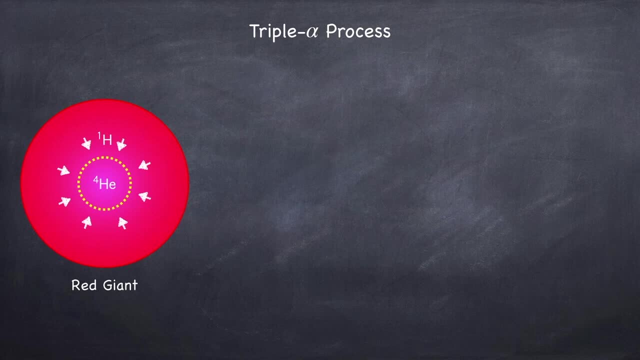 Helium fusion, called the triple alpha process, is exactly what it sounds like. We have three alpha particles that come together and make one carbon-12 nucleus, And in the process photons are emitted. We'll look at this process in further detail. 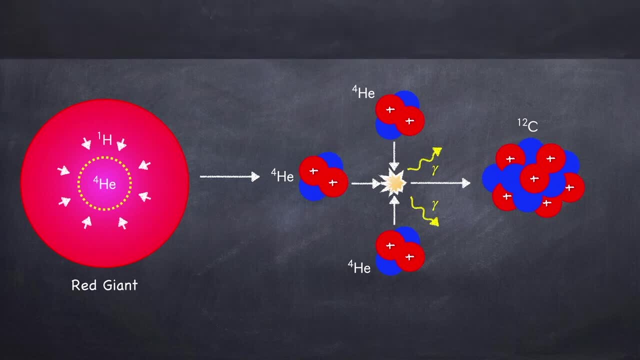 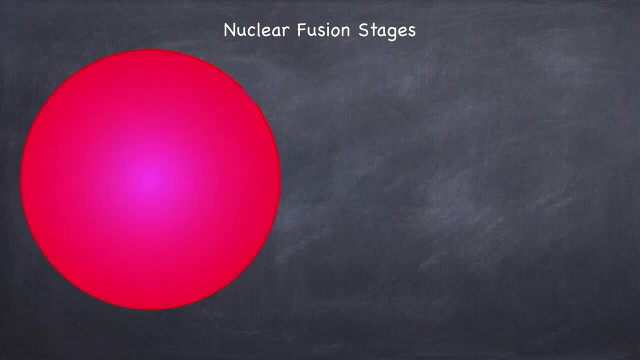 in a future video. Eventually, the core will run out of helium and the star will move on to the next nuclear burning phase. In all, we're going to have the following nuclear fusion stages Once the star's core runs out of hydrogen: 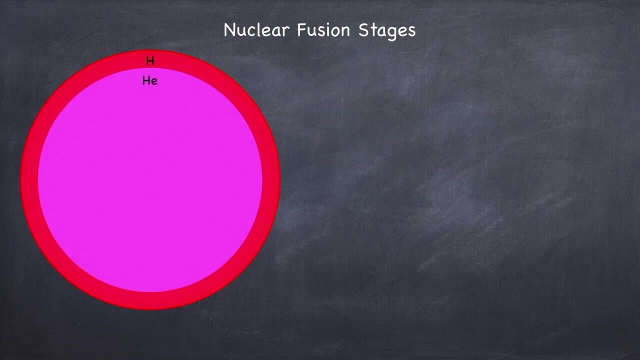 it'll start fusing helium, And so now we have a helium core with a hydrogen envelope. Eventually you run out of helium and you start fusing carbon. So now you have three layers. You've got a carbon core, then you've got helium outside of that. 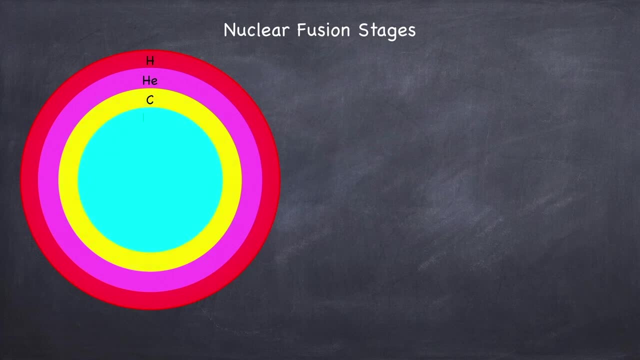 and you've got hydrogen outside of that. Next stage is neon, then oxygen, then silicon and then iron. This is somewhat of an oversimplification, As you don't go from only fusing hydrogen to only fusing helium, to only fusing carbon, etc. 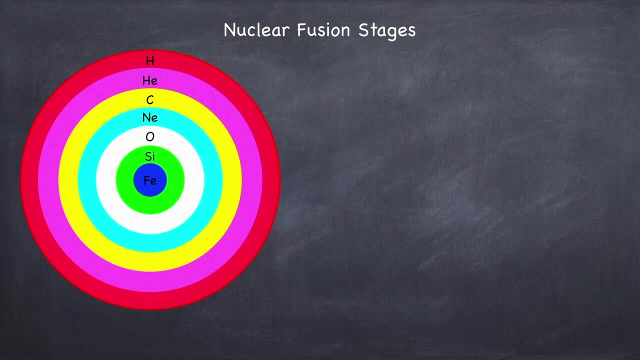 These envelopes really represent the dominant nuclear processes as well as the dominant nuclei left over in the envelopes. In reality, every kind of nuclear fusion has a chance of occurring, But as you move up the periodic table, the charge of each nucleus increases, increasing the electrostatic repulsion. 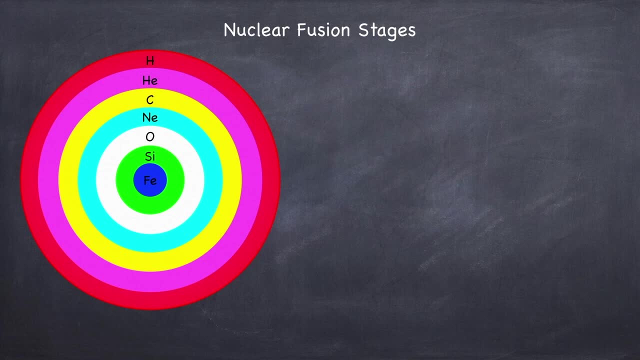 requiring higher speeds for fusion to occur. Therefore the nuclear fusion rates are temperature-dependent and a higher temperature is required at each nuclear fusion stage. Once you get to iron you can't fuse anymore. You can't go beyond iron. So at this point, 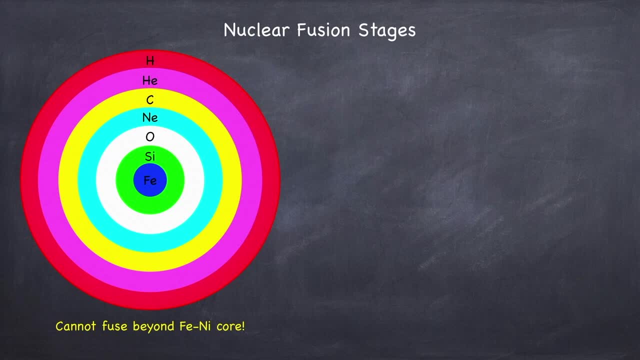 you're left with an iron-nickel core surrounded by these layers of envelopes corresponding to the previous nuclear fusion stages. Now you might not necessarily get to iron. The star has to be massive enough to get hot enough. If it's not hot enough, fusion will stall. 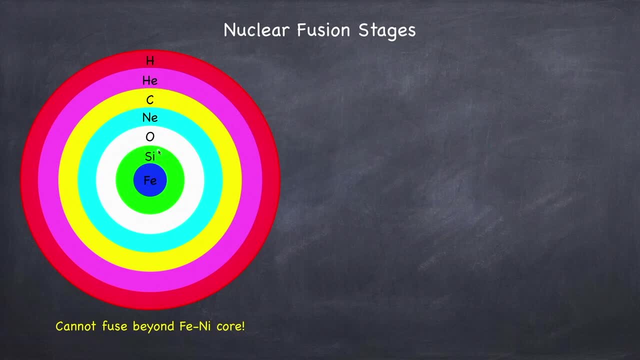 and you'll be left with what's called a white dwarf made up of carbon and oxygen and silicon, depending exactly on the mass and composition of the star. So why does this happen? Recall in Stellar Physics 1a, when we looked at the smallest mass a star could have. 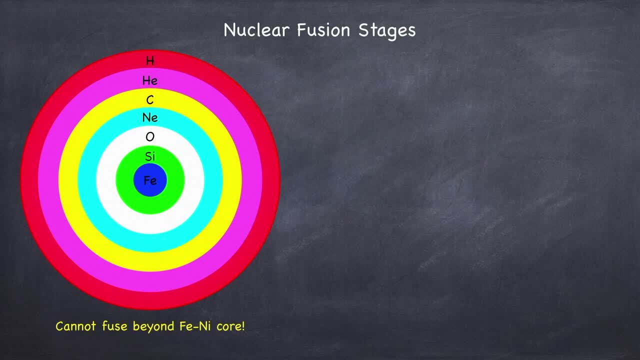 we discussed a quantum mechanical limit where at a certain density the temperature no longer increases with pressure. So if the star is not massive enough, it'll reach this limit, and now the pressure will increase. so the star will still be supported against gravity, but the temperature 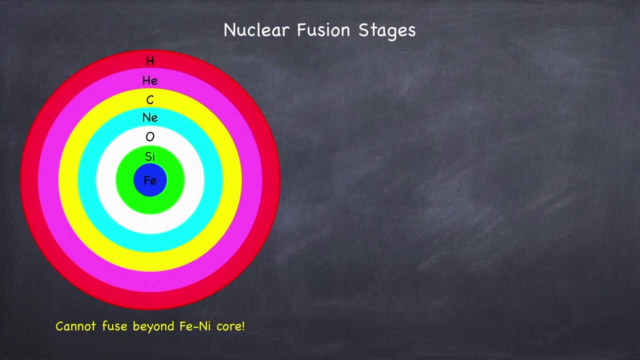 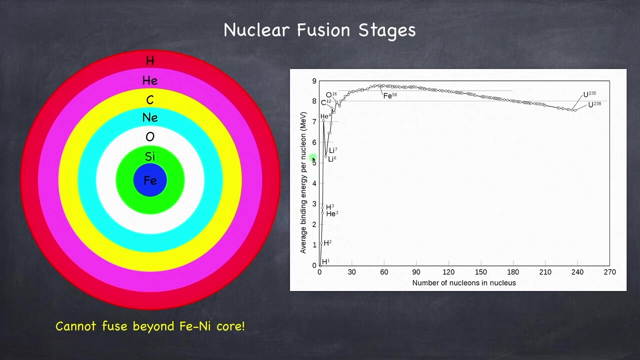 will not increase, And so it will still never get hot enough to go on to the next nuclear burning stage, And that's what we call a white dwarf. So why can't we fuse beyond iron? Here we have nuclear binding energy per nucleon. 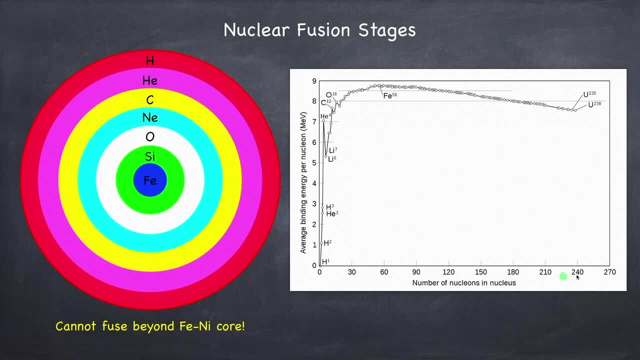 in units of MeV, and here we have the number of nucleons in a nucleus. We start off with hydrogen, which has a binding energy of zero. there's no binding energy for hydrogen. Then we have helium all the way up here at 7 MeV per baryon. 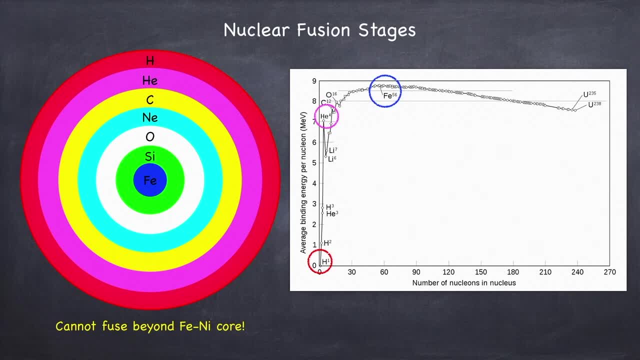 And here is iron, and notice iron-56 has the highest binding energy. After that, the binding energy decreases, meaning that in order to fuse beyond iron, it will take energy to do so rather than releasing energy. And so if you start fusing beyond iron, 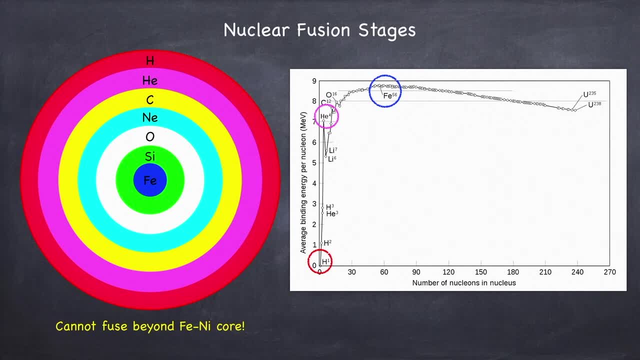 instead of releasing energy to support it against gravity, it will suck energy into the nucleons and the whole star will collapse. That's why, once you get to iron, the star will no longer have a source of energy to support itself against gravity and you will have 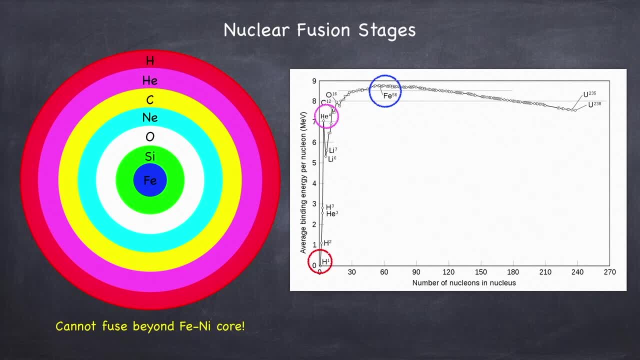 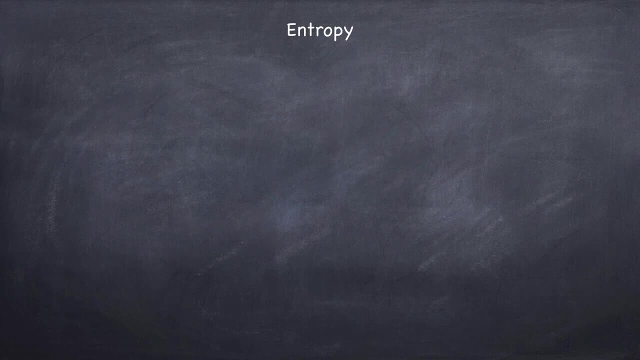 a core collapse supernova. Notice that even if you fuse all the way to iron, the bulk of the binding energy is released during hydrogen fusion. Now I want to discuss entropy, Because there's something very interesting happening here. Initially, the star is made up of hydrogen. 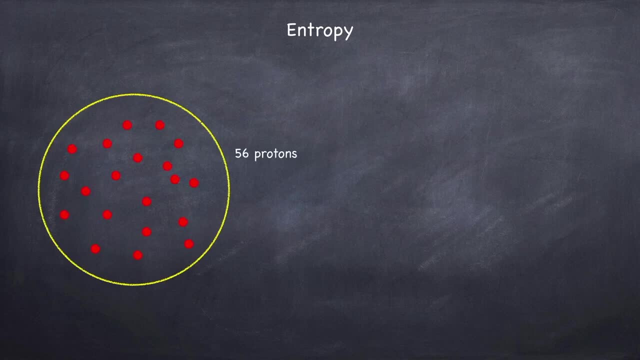 So let's say we have 56 protons. Eventually, if the star is large enough, these 56 protons will be fused into one iron nucleus. So you've gone from 56 particles in the system to one. In other words, we've gone from a high 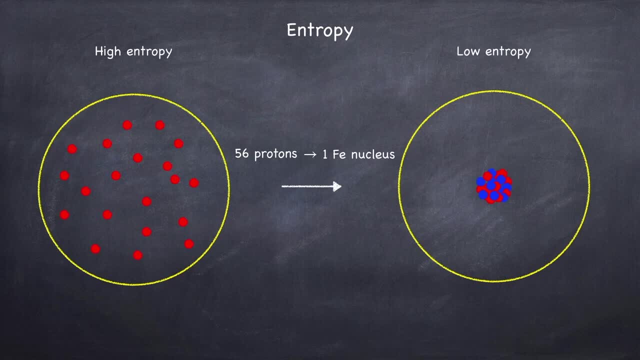 entropy state to a low entropy state, And this entropy is carried out of the star through neutrinos. Recall that neutrinos just leave the star, And earlier I said that they're basically just lost energy. But what's more important is that they carry out. 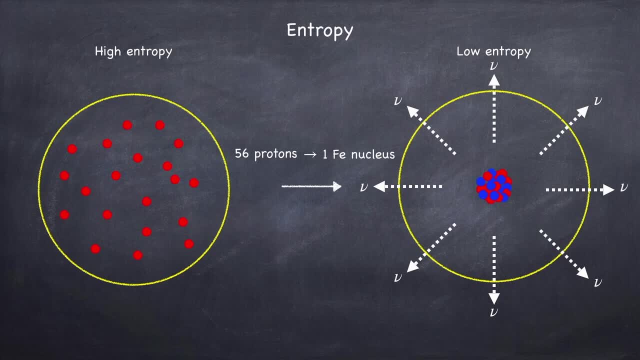 all of the entropy. So where are all these neutrinos coming from? In the star, photons and electrons are in thermal equilibrium. So you have this process in which two photons can create an electron-positron pair and vice versa, And since they're in thermal equilibrium, 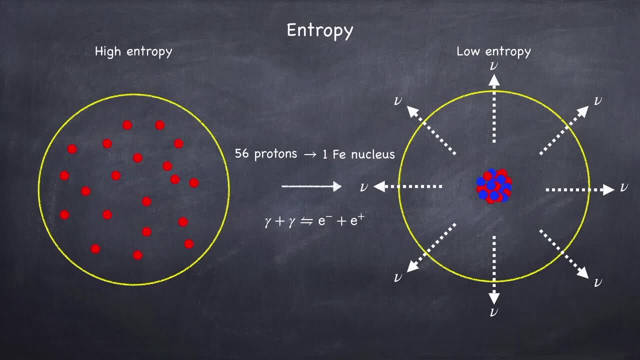 these rates are equal in both directions. Now, in the earlier stages of nuclear fusion, this doesn't happen very often, Because in order to make an electron-positron pair, the photons have to have at least as much energy as two electron masses. 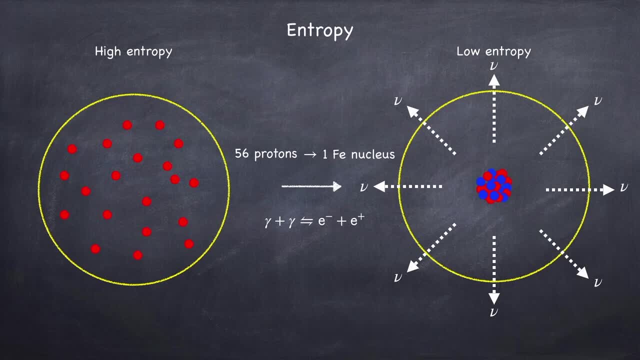 So the star has to be very hot for this process to have an appreciable effect. There is also the possibility that an electron-positron pair converts into a neutrino-antineutrino pair, And in that case the neutrinos are not in thermal. 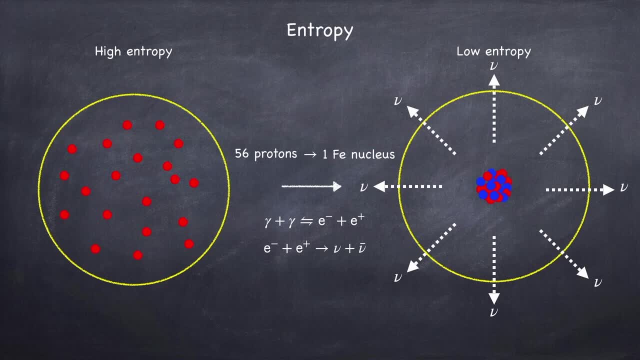 equilibrium with the electrons, and so this is a one-directional reaction. And so if you have a lot of electron-positron pairs around, occasionally they will make a neutrino-antineutrino pair, which will leave the star carrying out energy and more. 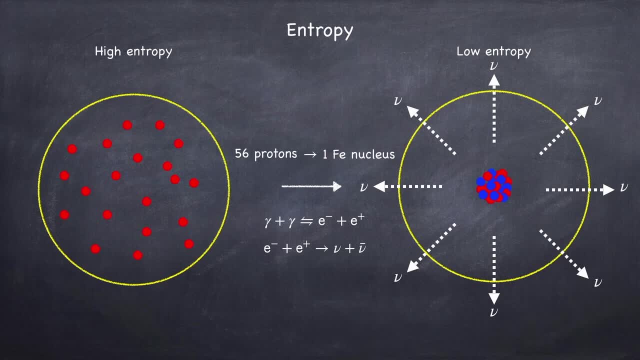 importantly, entropy. So what does this mean from a thermodynamic point of view? That stars go from a high entropy system to a very low entropy system, dumping their entropy out into space via neutrinos. In other words, stars are giant freezers. 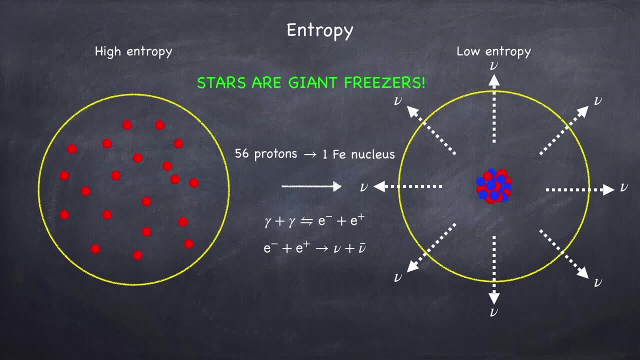 At least massive ones are. As a star goes from the main sequence, meaning its hydrogen burning phase, to a collapsing iron core, the entropy per baryon will go from about 10 units of Boltzmann's constant to less than 1. In fact, 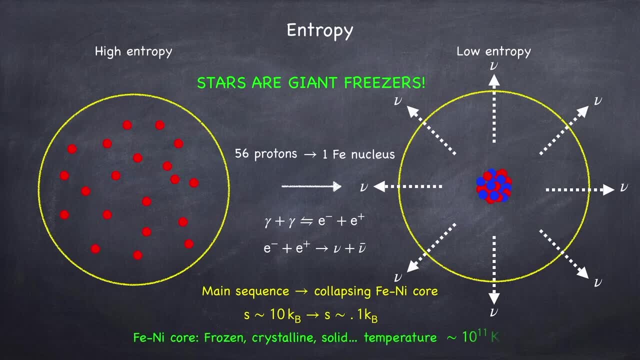 so much entropy is sucked out by neutrinos that the collapsing iron core of a star is a frozen crystalline solid with a temperature of about 100 billion Kelvin. We'll look at this in more detail further on down the line when we get to collapsing cores. 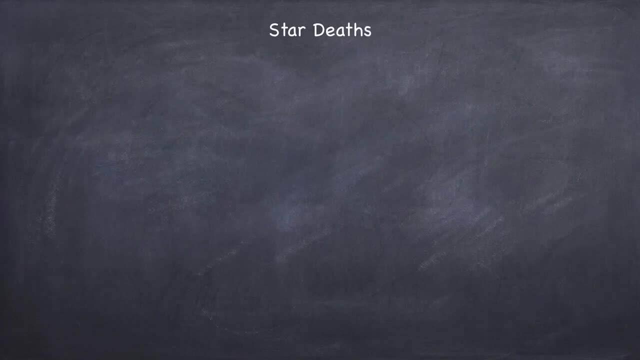 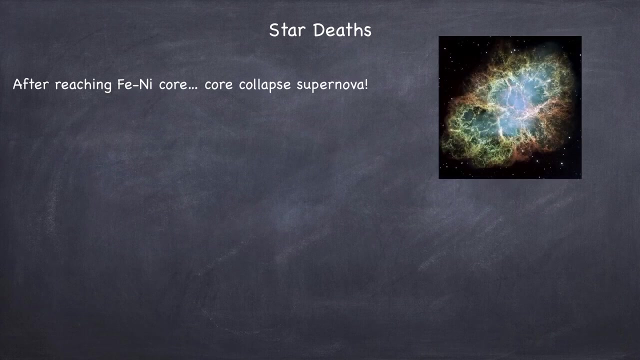 Now let's take a look at star deaths. As I mentioned, once the star gets to an iron core, it can no longer generate energy through fusion and you get a core collapse supernova. This will leave behind a remnant of either a neutron, 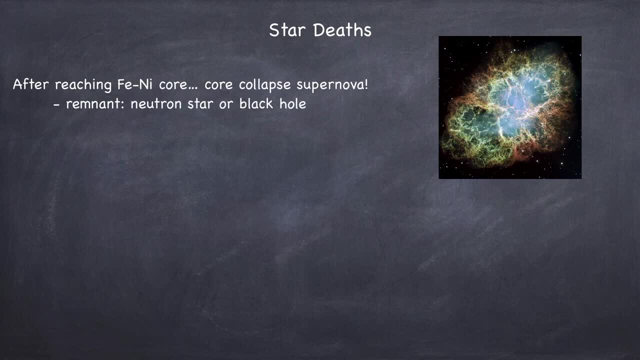 star or a black hole, depending on how massive the star is. So over here on the right, we have a picture of a supernova that went off. This is called the Crab Nebula, And in the center there's a neutron star. More specifically, 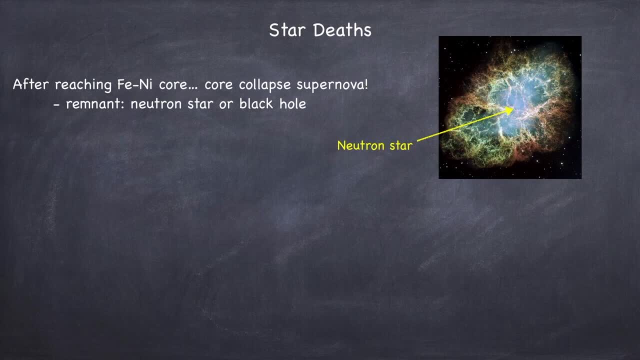 people call it a pulsar, but a pulsar is just a spinning neutron star. This only happens if the star can get to iron. If the star, however, is less than about 10 solar masses, fusion will stop somewhere between carbon and silicon. 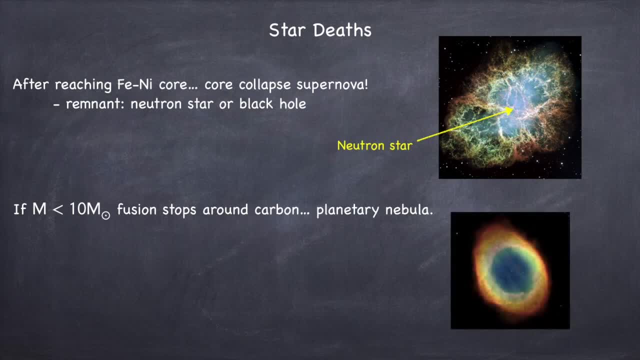 and it will shed its outer layers in what's called a planetary nebula and leave behind a white dwarf remnant. And the white dwarf may in the future explode in what's called a Type Ia supernova. This will happen if it somehow. 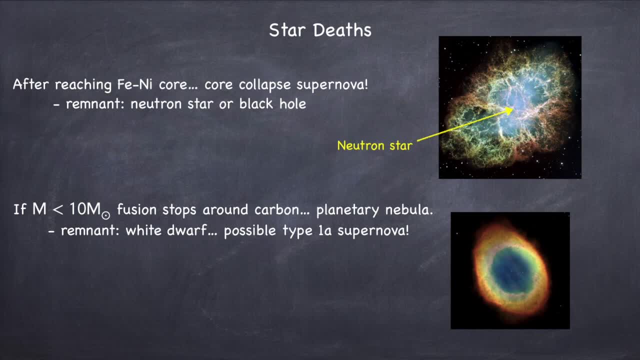 manages to increase its mass to more than 1.4 solar masses. The way this could happen is if it's in a binary system with another star and it starts sucking off material from the star. that material piles up onto the white dwarf it reaches. 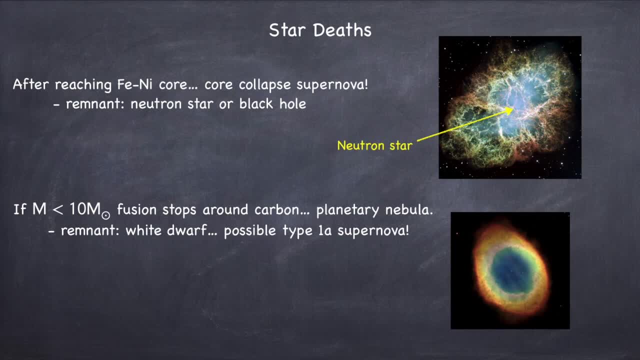 this mass limit called the Chandrasekhar limit, and it will explode. This is also something we'll eventually look at much later down the line. when we take a look at compact objects, We can now summarize the full life cycle of a star. 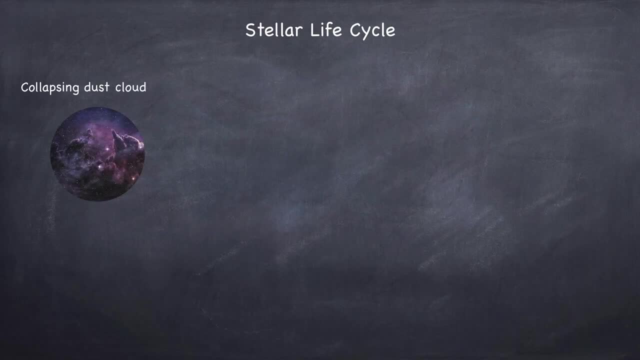 As we discussed in Stellar Physics 1a, you start off with a collapsing dust cloud. It heats up until it fuses hydrogen and now you have a main sequence: star. Once the star runs out of hydrogen in its core, the core will. 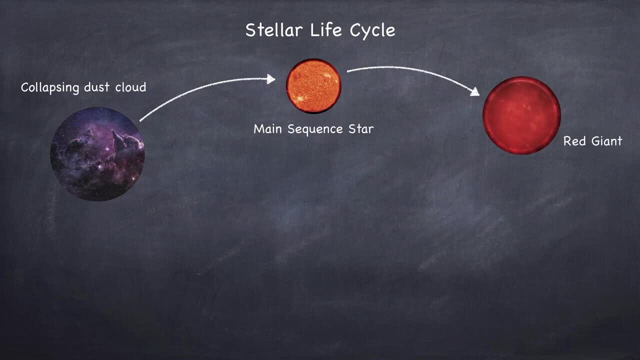 contract until it gets hot enough to fuse helium, at which point the outer layers of the star will expand and you'll have a red giant. Then there are two possibilities: Either it fuses all the way to iron, in which case you get a core collapse supernova. 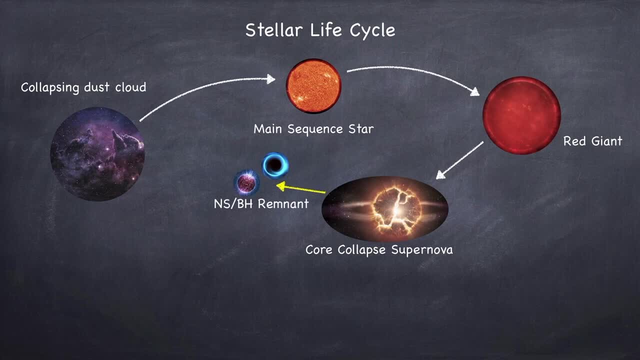 leaving behind either a black hole or neutron star remnant, and the material expelled in the supernova will eventually find its way into another collapsing dust cloud, and the whole cycle repeats. If, on the other hand, the star is not massive enough and 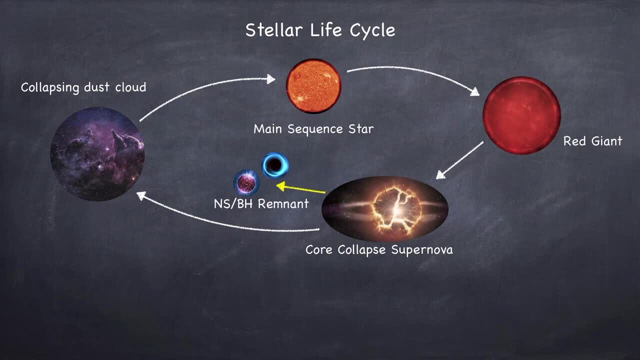 fusion is stalled somewhere prior to iron, it will shed its outer layers, creating a planetary nebula. I don't know why it's called planetary- it's got nothing to do with planets- Leaving behind a white dwarf remnant And again the dust.